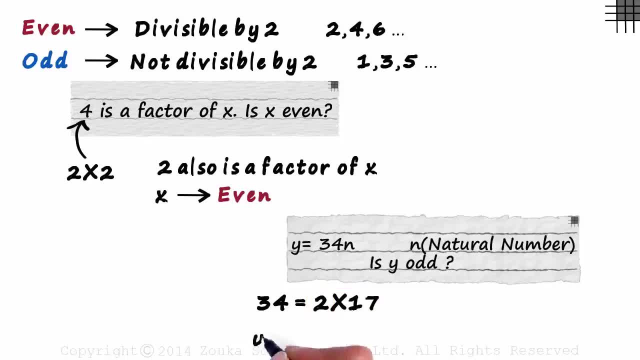 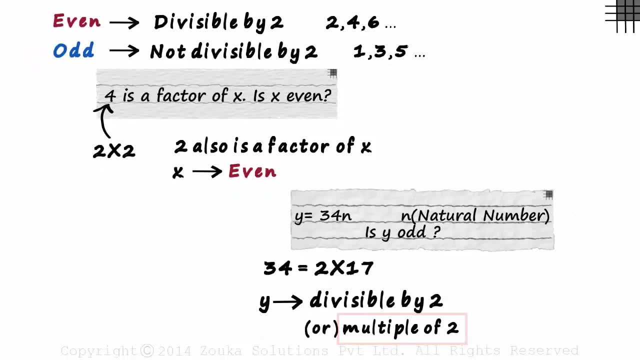 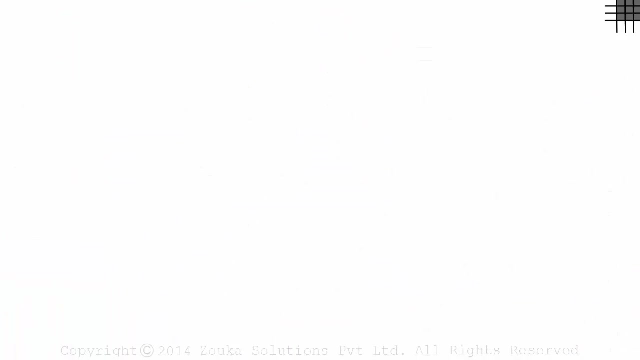 no matter what that something is, Y will surely be divisible by 2.. Or we can also say that Y is a multiple of 2. In any case, we can be sure that Y is even and not odd. Do we get special results when we add or subtract odd and even numbers? 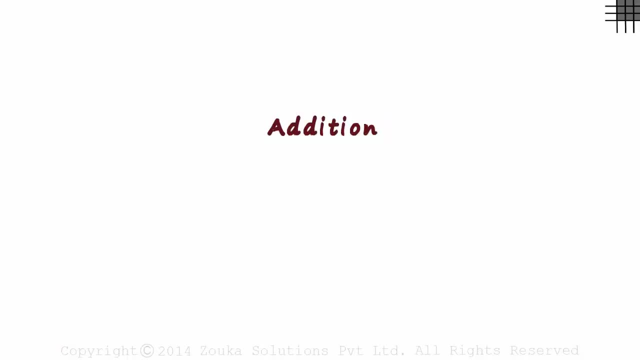 Let's look at addition first. Look at it logically. Only three cases can exist: Even plus, even odd, plus odd or even plus odd. For each of these three cases, the case is even plus odd. There can be three possibilities: We may get an even number or an odd number, or maybe get nothing specific at all. 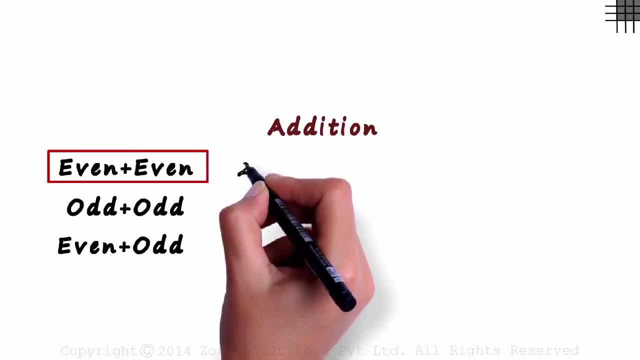 An even plus even, example, would be something like 2 plus 4.. Even plus even, We get a 6,, which is an even number. Let's say, we add 6 and 10,, which are even numbers, We get 16,, which is an even number. 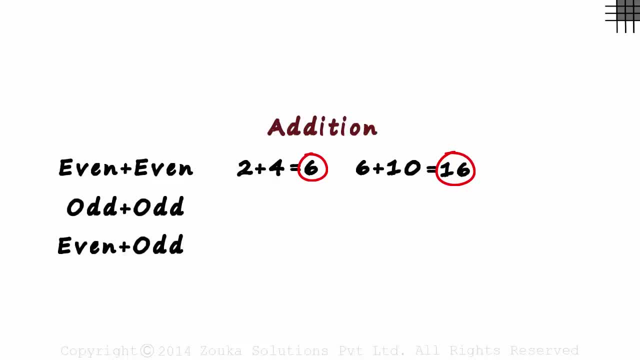 No matter what even numbers you consider, their sum will always be even. What about odd plus odd? Look at these two examples: One plus three and five plus seven. Both cases gave us an even number. Addition of odd numbers will also result in an even number. 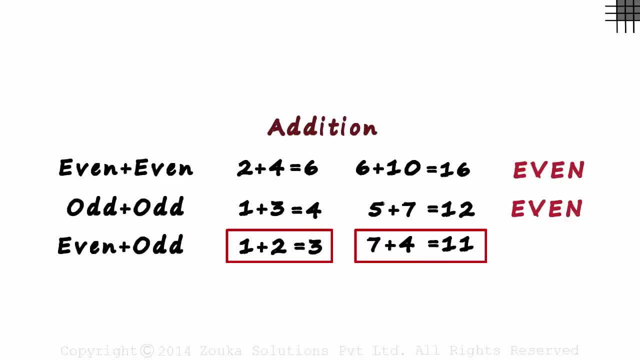 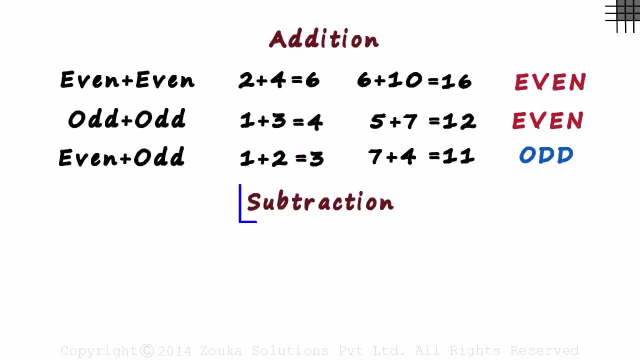 Even plus odd. Here are a couple of examples for even plus odd. Yes, Both result in an odd number. Will it be different for subtraction? For subtraction as well, there will be three cases: Even minus, even odd, minus odd and even minus odd. 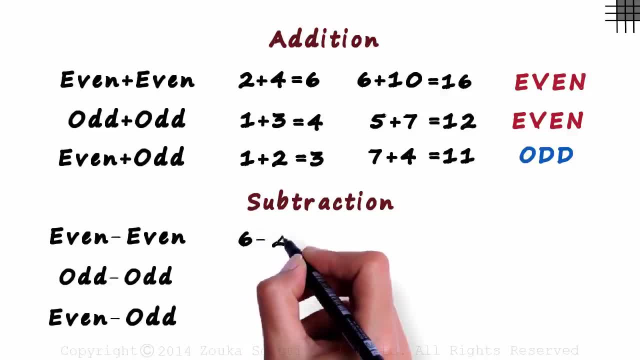 An example of even minus even would be 6 minus 2.. That gives us 4.. Or 12 minus 6,, which also gives us an even number. Even minus even will always give us an even number, And you can see that odd minus odd will also give us an even number.